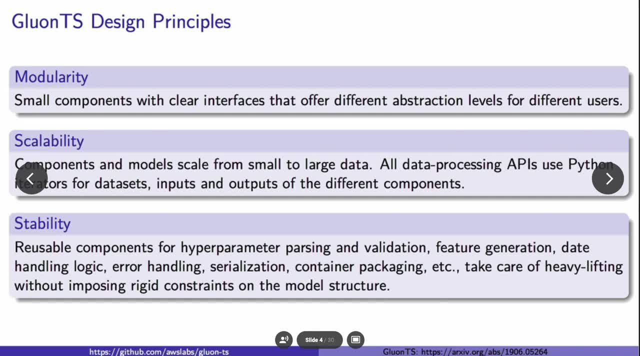 So one of our main uses is the Gluon-TS design principles. So one of our main uses is the Gluon-TS design principles. So one of our main uses is the Gluon-TS design principles, And the user base would be for scientists who want to build new models. 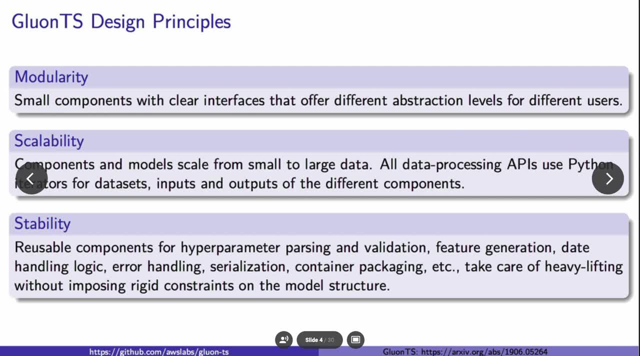 So here we have small components that they can use to develop these models, as well as it's reproducible, which gives a very flexible framework for scientists. In particular, you can use a log file to define your configuration and parameters and rerun the experiment from that given log file. 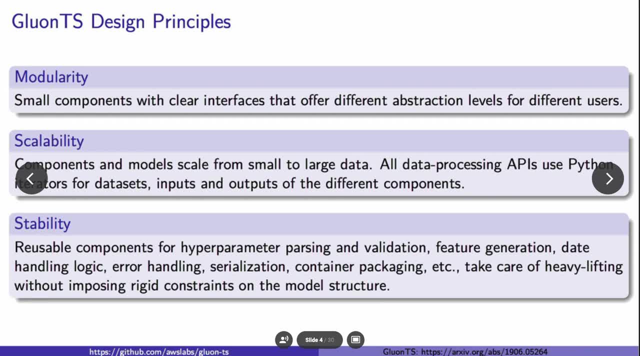 On the opposite end of the spectrum from scientists, who we also like to support, would be practitioners who just want to use an out-of-the-box model. So we also provide baseline models with ASD. So we also provide baseline models with ASD. So we also provide baseline models with ASD. 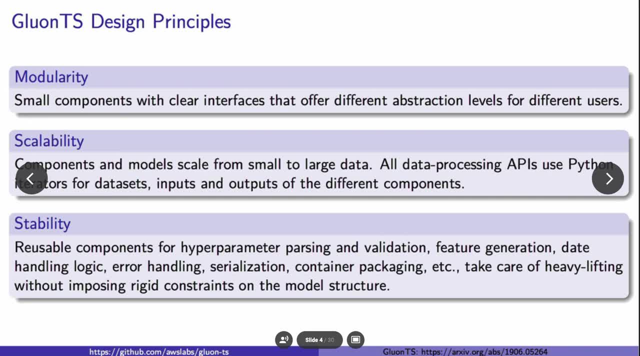 the package. second, it's scalable, so we've designed it to have models and components to scale from small to large data sets. in particular, all data processing apis use python iterators for data sets, inputs and outputs of the different components, and it's also stable. we have reusable components. 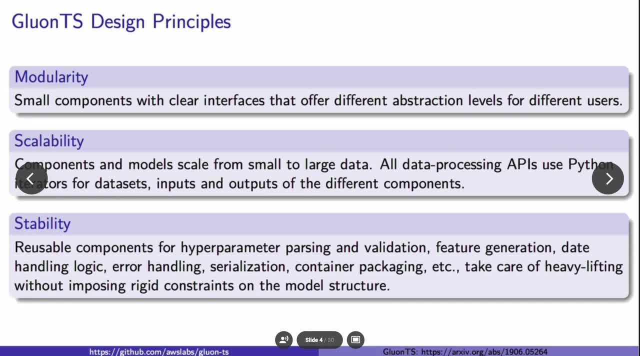 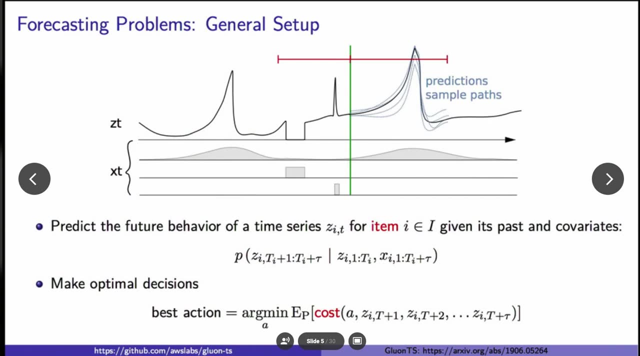 for hyper parameter parsing and validation, feature generation, date handling, logic, error logic, serialization, container packaging, and these help take care of the heavy lifting for you without imposing rigid constraints on the model structure. so let's go over the general problem. so here you'll see plotted. we have a univariate time series, the observations are given by zt and the input 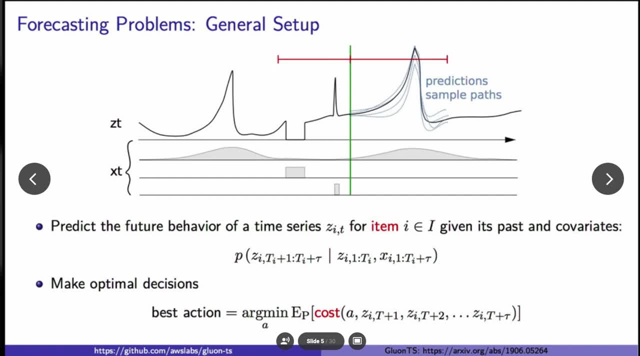 covariance are given by xt and the x-axis. here is time. so what are we trying to do in forecasting? we're trying to predict the future values, in particular for a given item i. we want to predict the values in the future up until forecast horizon of tau. given the past observations, as 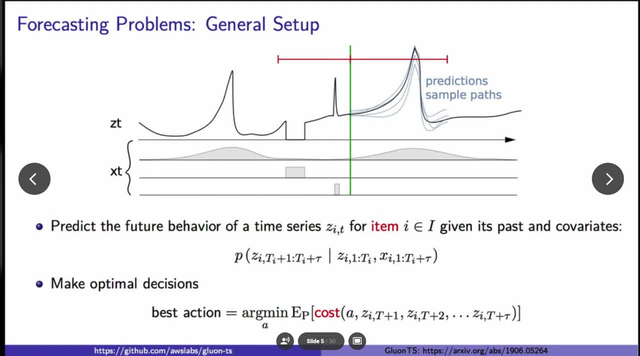 well as all of the covariance, and we hope to use this forecast to be able to make optimal downseams decisions, which we'll see by the second equation. so our library is not only supports forecasting methods but also time series methods in general, in particular smoothing for missing value implementation. 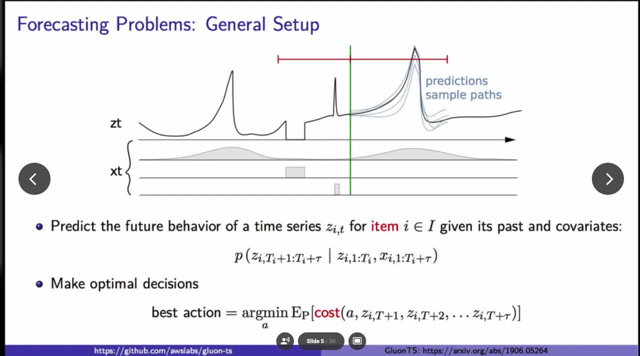 and anomaly detection. so in missing value invitation you're also trying to learn a joint distribution over zi t and at that point the time values are not necessarily in the future. they could be at any arbitrary time at which you have a missing value. similarly, an anomaly detection you want. 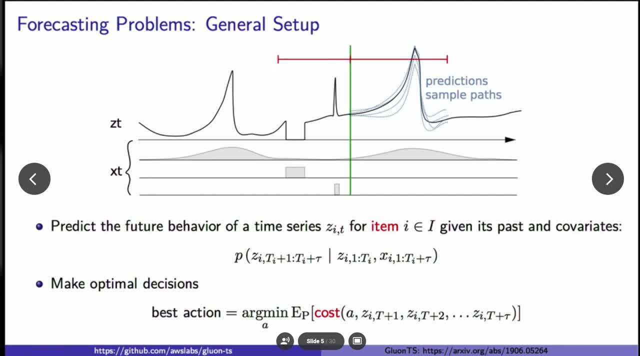 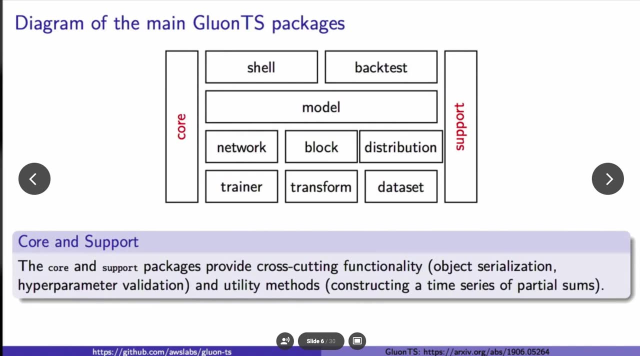 to find the corresponding observations at the points where you have anomalies so we can think about. in general, this library could be used to solve anything that would like to predict a joint distribution at arbitrary points in time. and here we have a diagram of the main parameters for table two and table three and table four. you can see at table three that the 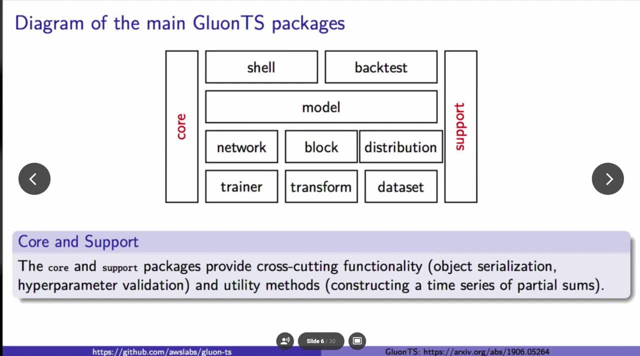 lower right hand corner. the orders of order are given by the set of a set of values that are the reduction of value in terms of the total amount of data we want to achieve. i'm going to highlight a couple of these. i'm going to highlight a couple of these. 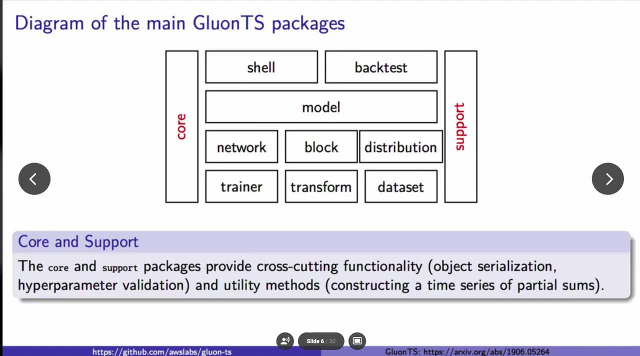 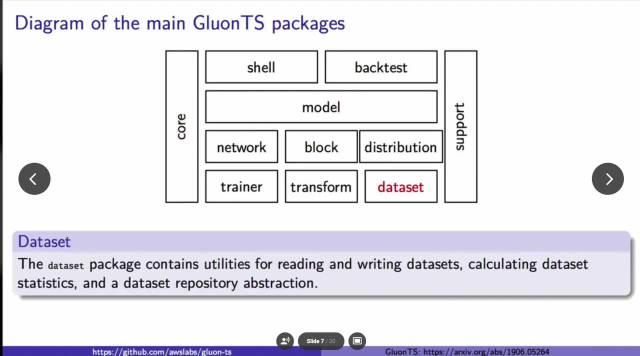 so first we have core and support packages, which are going to provide functionality for object serialization and hyper parameter validation, as i mentioned earlier, as well as utility methods. Another package we have is the data set package, so this would be one package that you would start with. 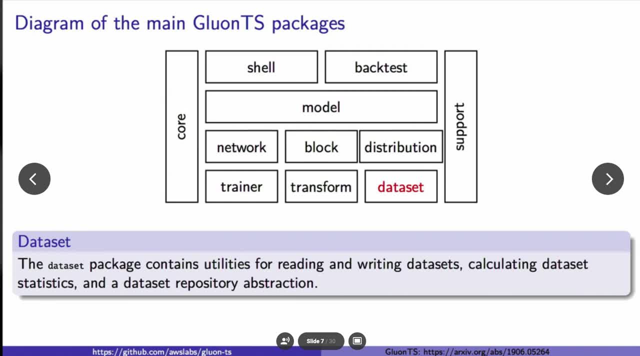 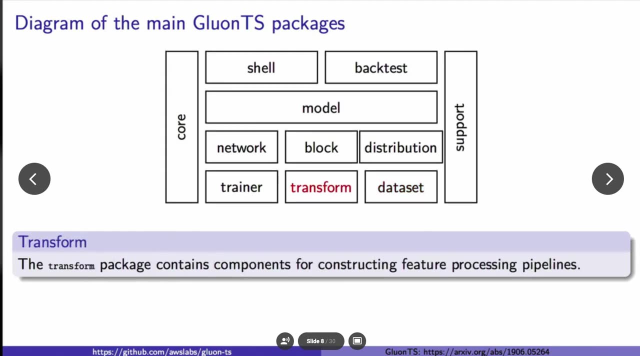 This will help you load your data and analyze your data. So here we provide utilities for reading and writing data sets, as well as calculating data set statistics, and it gives you a data set repository abstraction. So we make a data set loader class which consists of Python iterators. 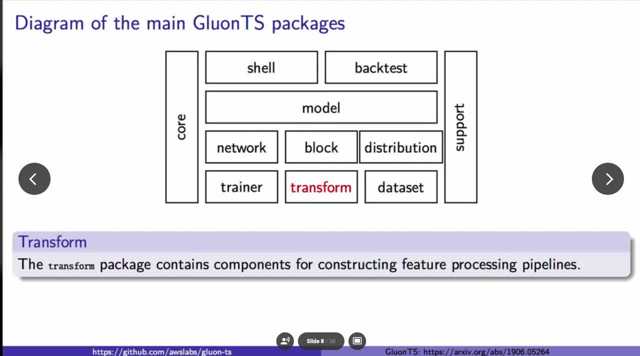 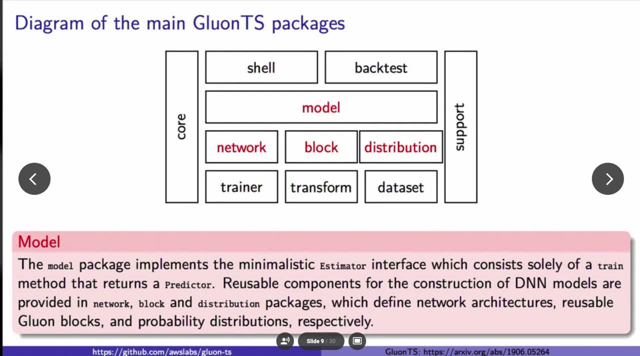 The transform package is used to do your feature processing pipeline, and we'll see examples of this later. One of the most important packages would be the model package. So here you'll see that you'll implement an estimator interface which will inherit from our base estimator class and you'll define a train method that will return a predictor. 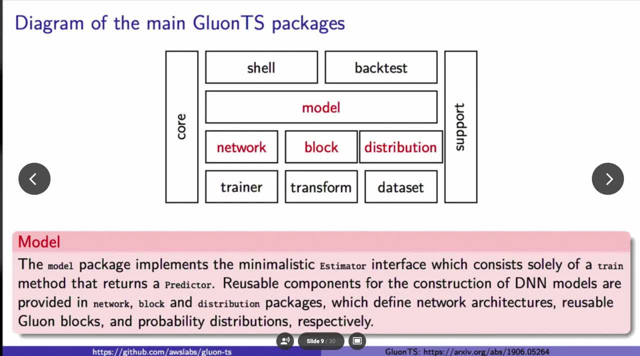 The predictor will then be used to evaluate your metrics and also plot your forecasts. So within this model we have reusable components for construction of other data sets. We have other neural network-based models and those are provided in the network block and distribution packages. 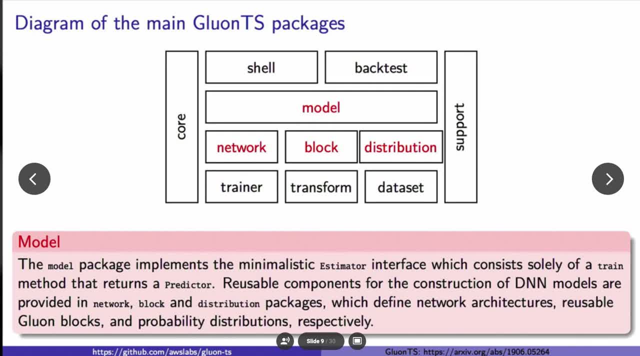 So the network package defines network architectures In block. we have reusable gluon blocks, so you'll see that gluon-ts is written in symbolic hybrid forward gluon form, And we also provide a probability distributions package, So this is almost a standalone package that you can use for different probability distributions. 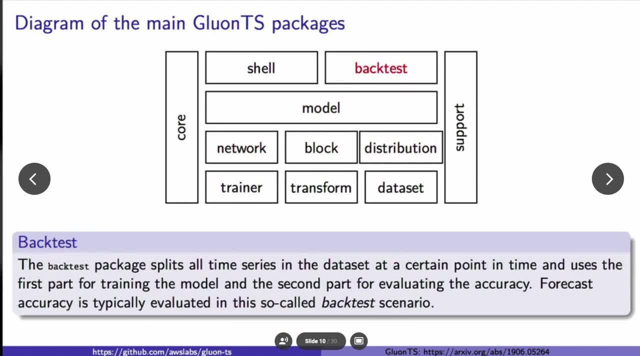 So Okay. So, lastly, you'd like to be able to evaluate the accuracy of your forecasting models, And how do we typically do that? That's with backtesting. So we also have a backtest package that will split all time series at a specific point. 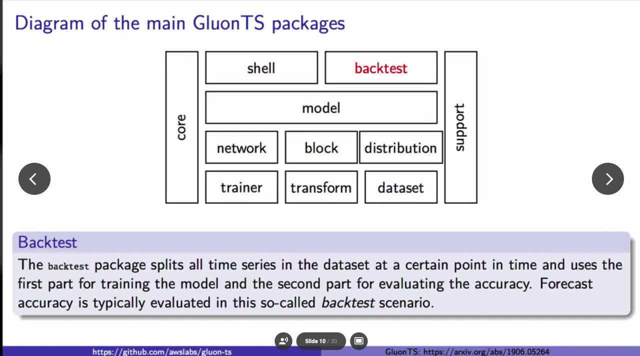 in time and use the first part for training- your model- and the second part for the evaluation. So if we think back to the picture, everything to the left of the green line would be your training set and to the right in the future would be your evaluation accuracy. 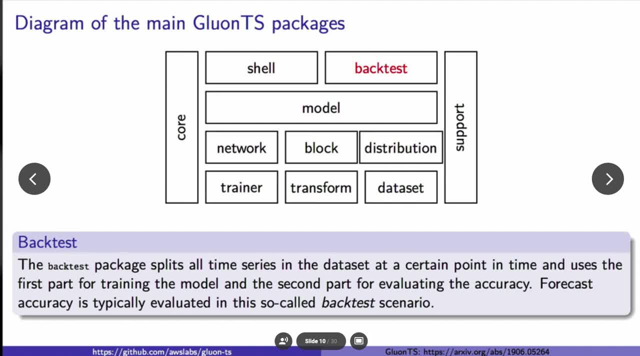 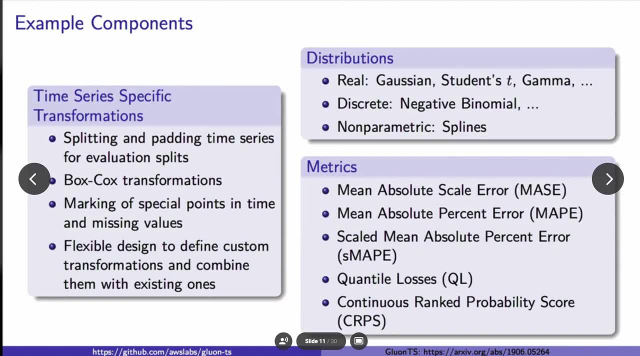 And we provide simple backtesting as well as more complicated scenarios such as rolling evaluations. So now that we've seen it at a high level, let's look at what are the example components of these. So, for example, for the time series transformations, we provide splitting and padding of time series. 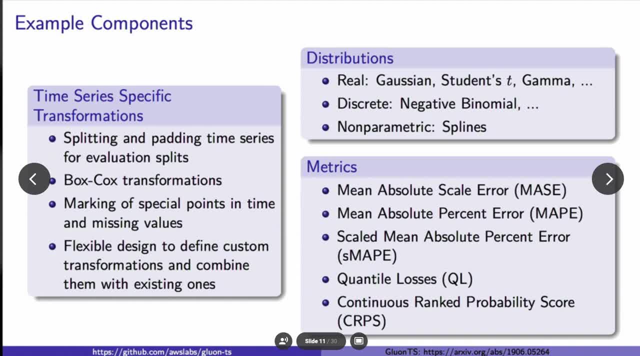 for evaluation splits as well as the box clocks transform. You can also mark special points in time and missing values. Most importantly, we have a flexible design for the user to define custom transformations, So you can define your own Future processing transformations, as well as combine them with existing ones, provided 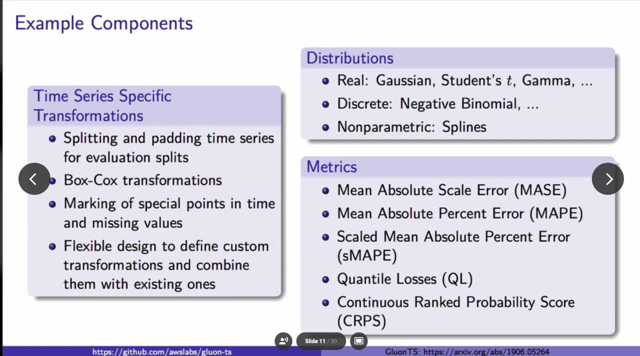 in the package. In terms of our probability distribution library, we provide real parametric distributions, such as single variant and multivariate Gaussian students, T gamma distribution and Laplacian distribution. For the discrete distributions, we also have negative binomial and we also provide non. 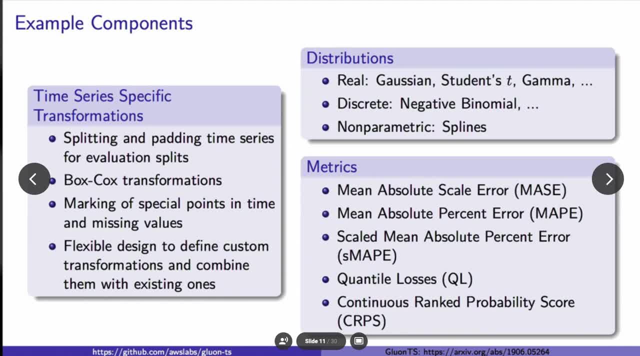 parametric distributions such as splines. in our backtesting scenario we output several different metrics. So, for example, we have the mean absolute, scale error, the bait metric and also the scaled mate, as well as the quantile losses. So the output from our models are probabilistic forecasts. 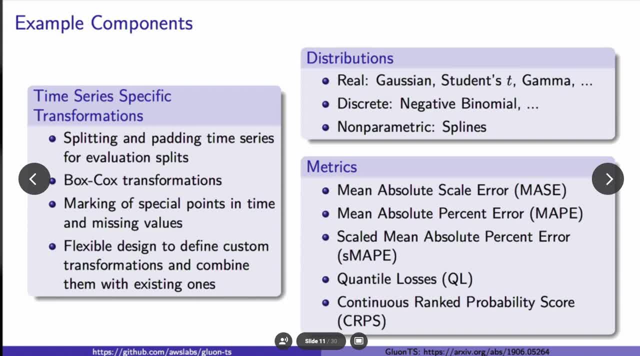 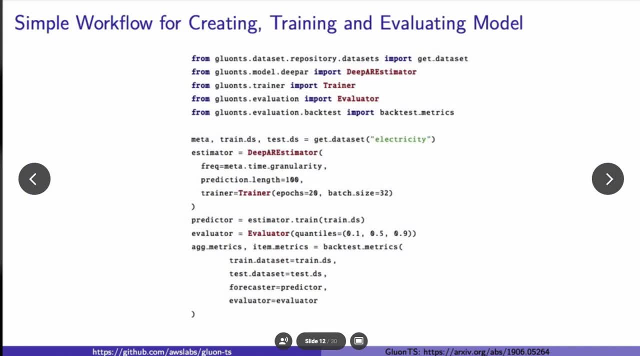 So quantile losses can be useful in evaluating these as well, And we provide the weighted and unweighted form as well as the continuous rank probability score. So now let's look at a sample piece of code here of how you can actually use glue on TS. 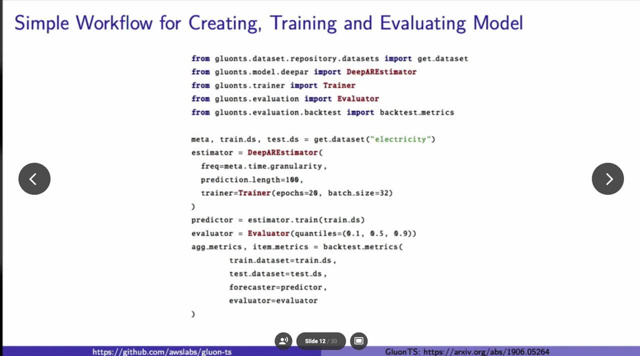 So you see, the first thing you want to do, What you want to do is load your data set. So we call the get data set routine on electricity, which is an open source data set from UC Irvine which is provided in glue on TS as well. 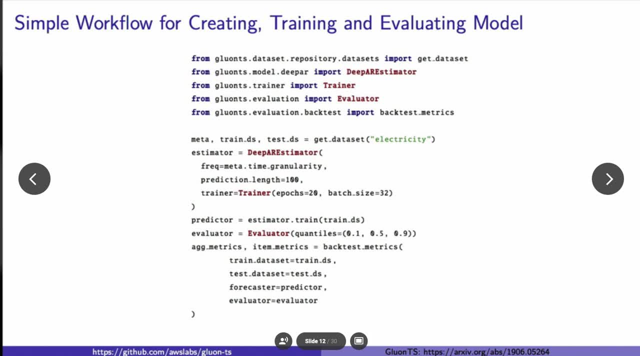 You'll see, it has three outpoints: meta, train DS and test DS. So meta contains all of the meta information of your data set And the training and tests provides the split data set for you at that particular time point. Here, you'll see, we're calling the estimator, which is our model. 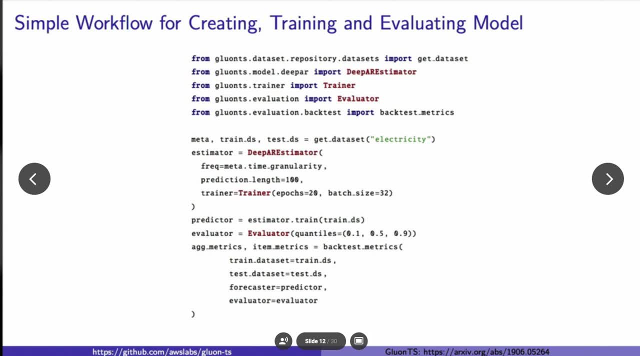 So we're using the built-in DeepAR estimator. So we're going to call the estimator, which is our model. So we're using the built-in DeepAR estimator And it's taking these three parameters as input. We can provide the frequency which is given in the metadata under the time granularity. 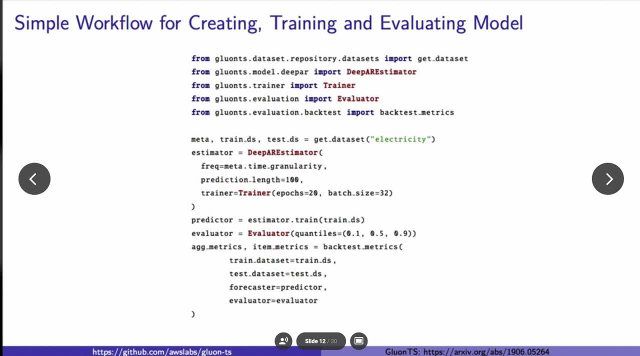 for you, And prediction length will just be: how far in the future do you want to predict, namely your forecast horizon, as well as a trainer. So here you'll see, we have a built-in trainer class which handles the stochastic gradient descent optimization for you, as well as the back propagation. 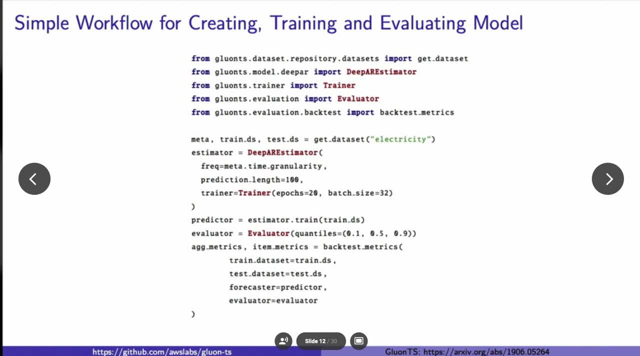 And you can define the optimization parameters that you'd like to pass into the trainer here. So here you'll see, in this example we're doing the optimization of a current parameter, doing the optimization over 20 epochs, which about with a batch size of 32 batches per epoch. 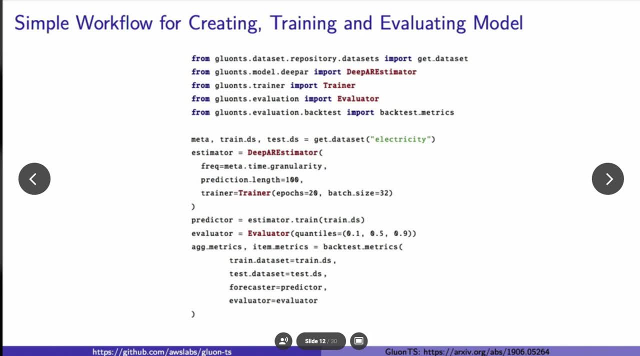 and you can also specify the step length, any optimization parameters you would like here. so once we have our estimator, we can call the train method, since that's defined for every estimator, and get our predictor. with the predictor here we're going to compute the back test metrics. 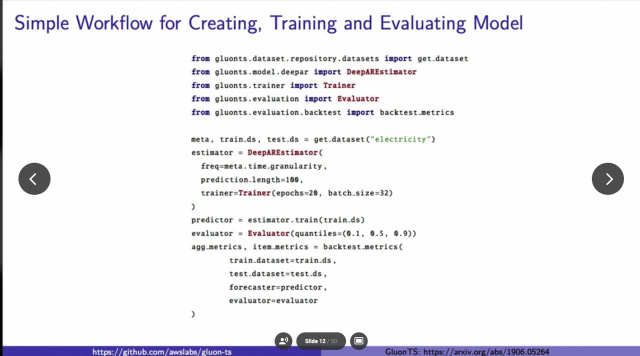 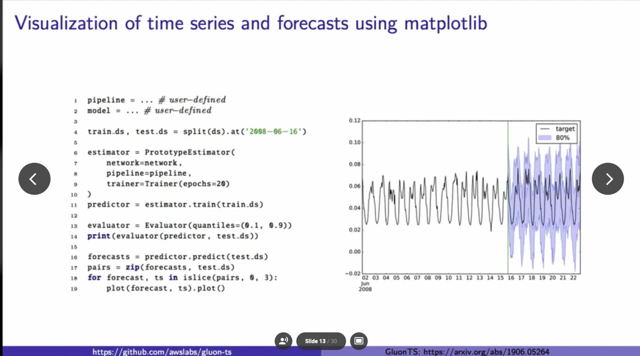 so in particular you'll see, we're computing the p10, p50 and p90 quantile loss here and the output of backtest metrics is going to give you the aggregate metrics over all your items as well as the item level metrics in this other example. here you'll see another excerpt of code. 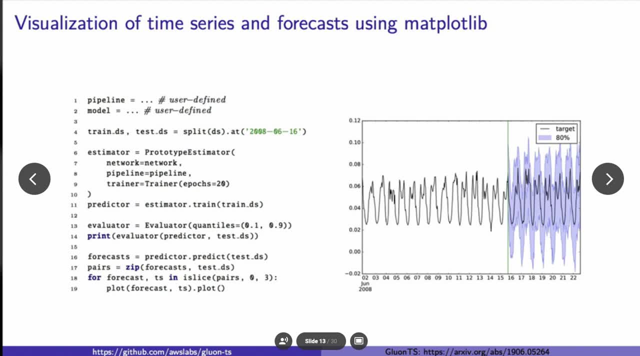 here we're using the train, defining the train and test split at a particular time point. but what i wanted to highlight here is you can also plot your forecast using matplotlib, which you'll see with the last line of code. here you can just call dot plot and on the right you'll see the plot. 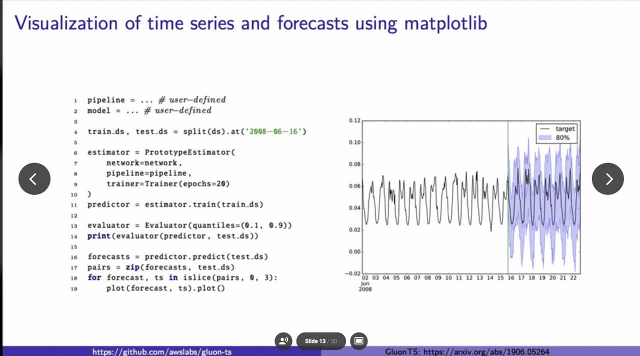 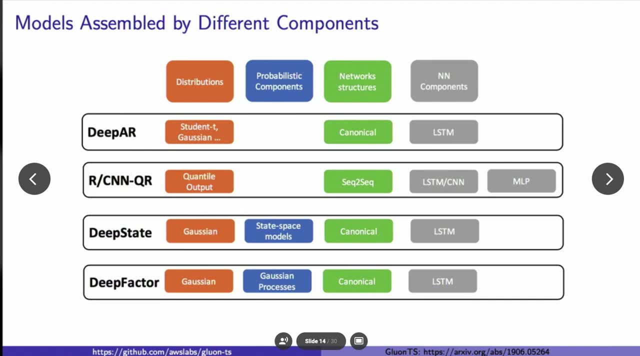 realistic forecasts, as indicated by the light blue region there. So now let's talk about the models that are a part of GLUON-TS and how they're assembled by the different components. So one of the main ideas of this slide is that we've built 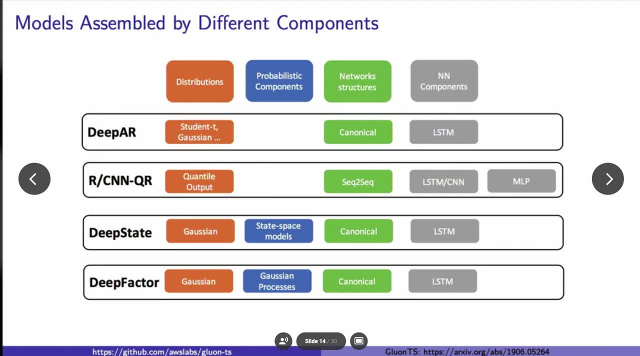 specific models for the user to use out of the box. but you can also use the given components to build your own models. So, for example, we can think of DeepAR as being a combination of using the distributions So you can define your own distribution. We have student T or 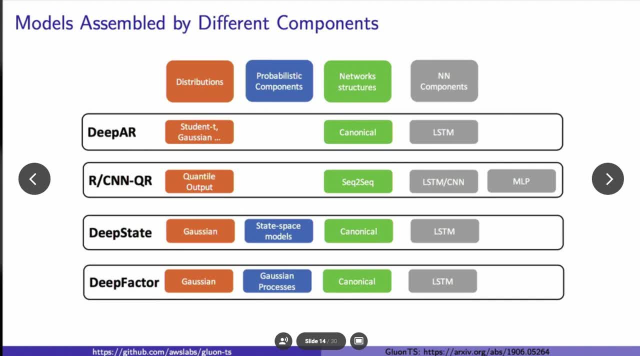 Gaussian or negative binomial combined with the canonical network. Our CNN-MQR is based off of NQRNN and that's composed of the quantile output distribution and sequence to sequence. The last two are newer methods: Deep State and Deep Factor. 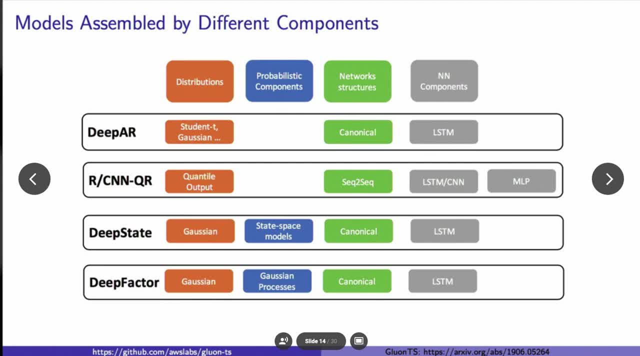 So these are combinations of classical neural network-based models with local models, and these are to come, And I just wanted to highlight that these are composed of probabilistic components and a canonical network. So, looking at these methods in a bit more detail, we'll see. on the left we have state-space. 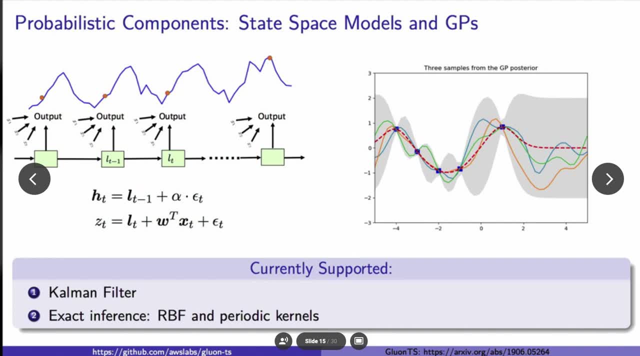 models. So in a state-space model you're trying to calculate the probability of the latent state, LT given LT minus one, and you have a state-space equation And then you'll use that to calculate the probability of ZT given LT. So classical models for time series: 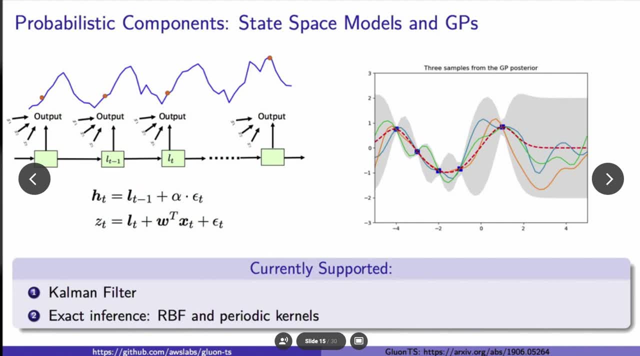 forecasting, such as ARIMA and ETS, could be placed in the state-space model format for a specified transition equation. So we provide this flexibility and a Kalman filter for that. On the right, you'll see we also support Gaussian processes. You can use that as out-of-the-box Gaussian process solver. 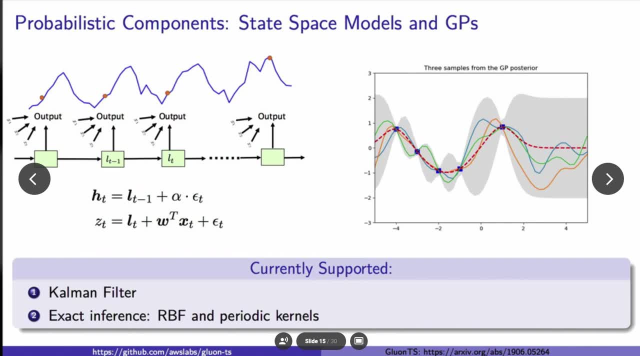 and also for time series specifically. So on the right you'll see we start with five blue data points and these are three samples from the Gaussian process, posterior plotted, as well as the uncertainty region plus or minus one standard deviation in gray For Gaussian processes. we support exact inference with RBF and periodic kernels. 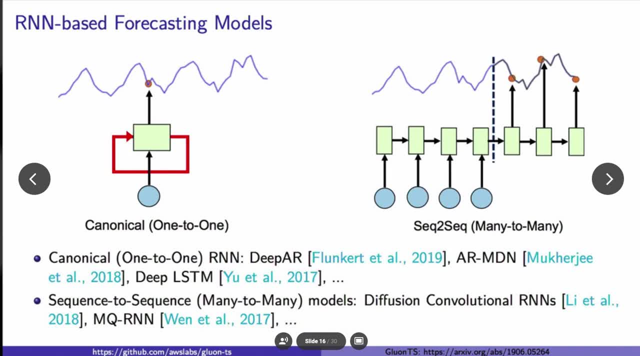 So let's get to the RNN-based forecasting models. So we can break them up into two categories. We have the canonical, which is one-to-one. We have one node going to one hidden unit, versus sequence-to-sequence, which you can think of as many-to-many. We have many nodes. 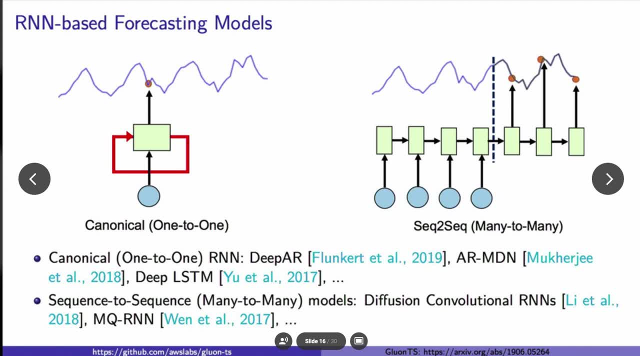 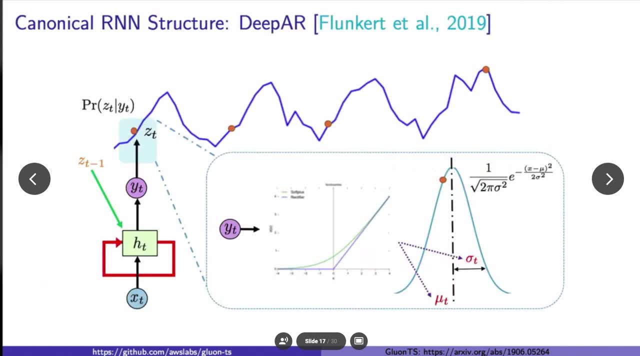 going to many hidden units, And here we're going to highlight DeepAR as a canonical example and MQRNN as a sequence-to-sequence example. So here you'll see DeepAR, and we provided the reference for more information, But here we have a canonical network where we're taking one node to one hidden unit. 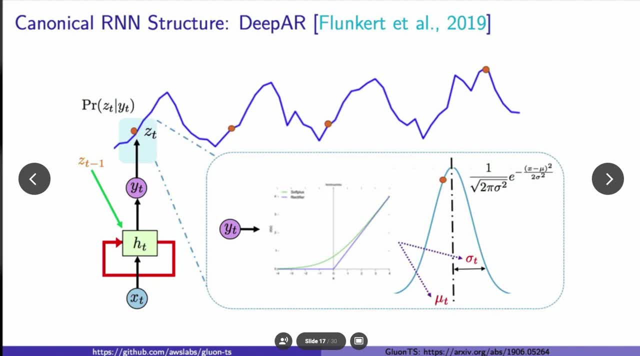 and here YT is going to be given by a parametric distribution, So what we need to do is estimate the parameters of this parametric distribution. In this case we have a Gaussian, so we need to learn the mean and standard deviation. You can also make DeepAR go distribution-free. 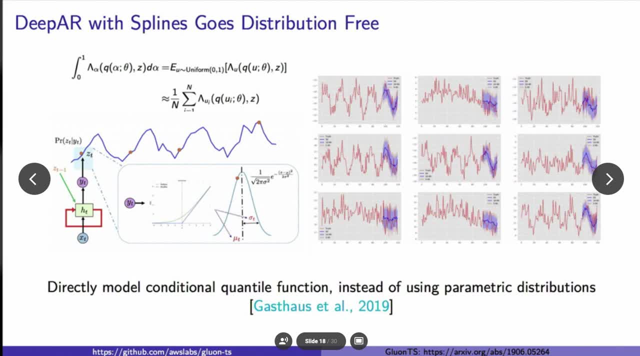 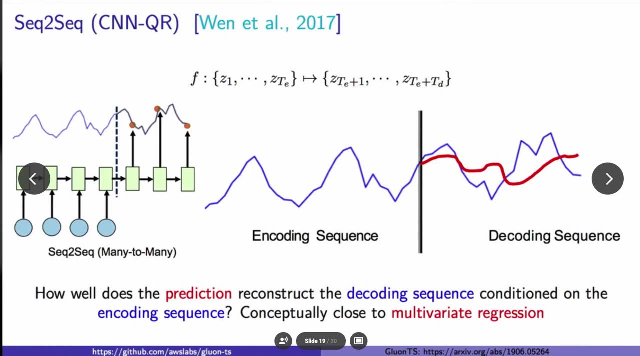 by utilizing splines. So here we can directly model the conditional quantile function instead of using parametric distributions. So here's an example of a sequence-to-sequence model now, which you can think of as an encoder-decoder model. So how well does the prediction reconstruct the decoding sequence, giving an encoding? 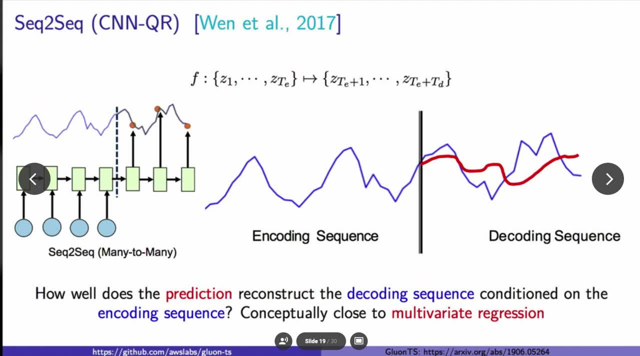 sequence And we see that this is similar to multivariate regression. So within GLOM-TS we provide a flexible sequence-to-sequence framework so you can even build your own sequence-to-sequence models Here we provide CNN-QR, which is a variant of MQRNN defined. 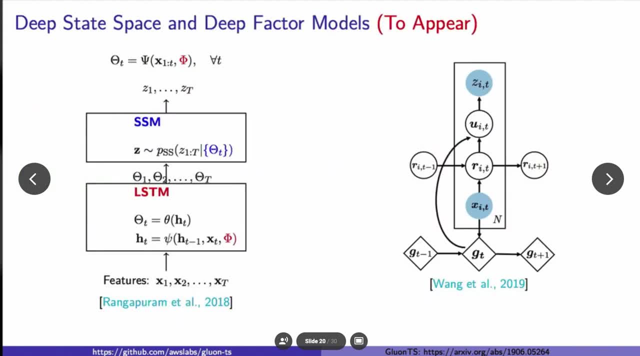 in the above paper And these are exciting future models to appear. Deep state space was a model that we developed at NIPS this year, and DeepFactor was actually a paper here. And what do these do? They combine neural networks with classical approaches, So you can think of DeepState as taking a 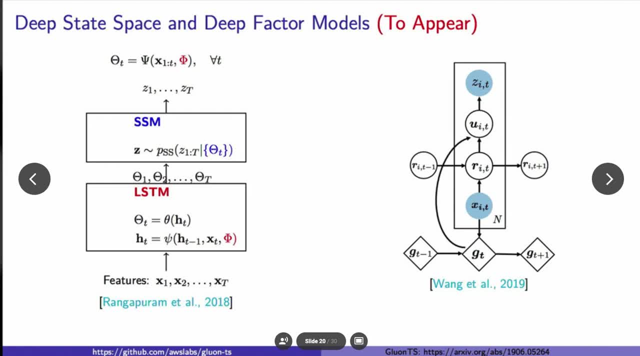 state space model and parameterizing it with a neural network, And in this case we support common filters and LDS for that. On the right you'll see DeepFactor. These diamond-nosed GT are the fixed-space models. They're the ones that we're going to use to predict the 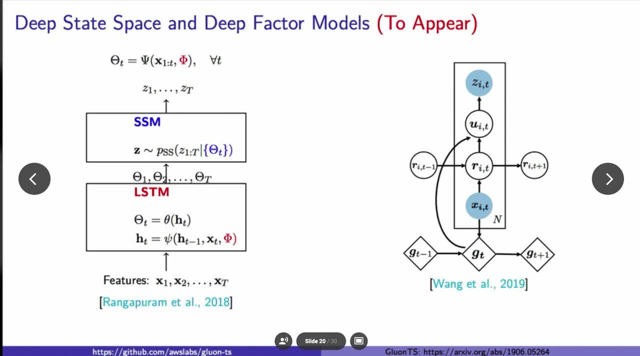 data. The RIT are the fixed effects as output from an RNN, and RIT are going to be a random effect. So these are the local model that will fit one time series at a time. Then your latent function, UIT, is going to be a sum of your fixed global effects from the neural 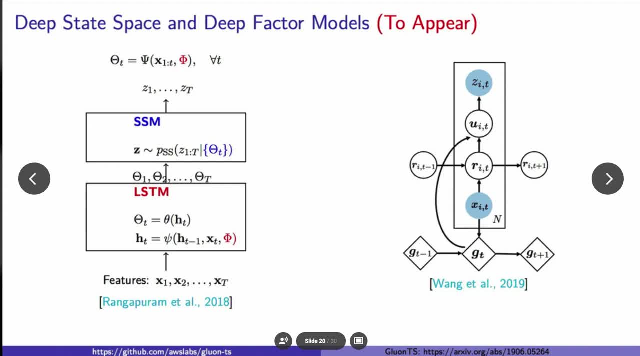 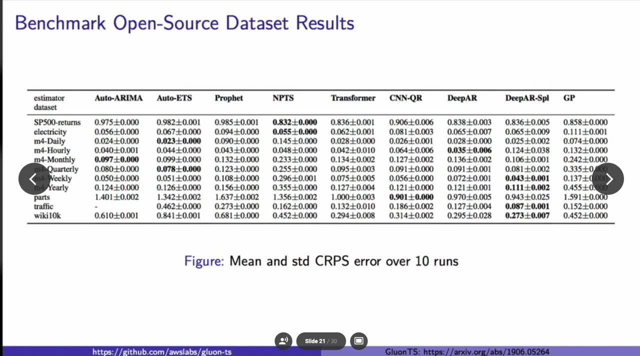 network with the local effects there And, for example, these RITs could be a Gaussian process within GLOM-TS. And then I also wanted to highlight: we benchmarked open source data set results across all the methods that we had in the data set, So it's important to keep that in mind. Here's the 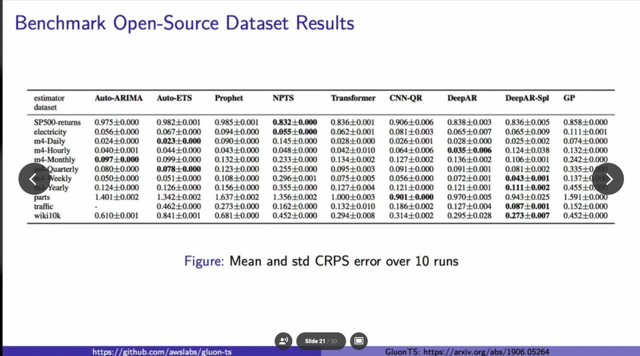 have within Glue-on-TS, as well as comparing to the classical methods within the R forecasting package. So here you'll see on the left: auto-REMA and auto-TS, which are part of the R forecasting package, are also available through Glue-on-TS, as well as Facebook's profit open source method. 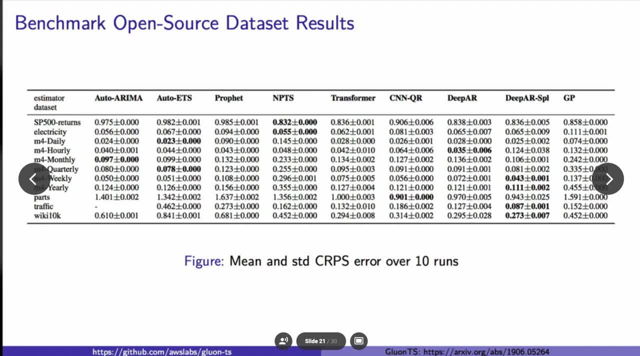 which is a Bayesian-based method, And it also highlights other methods that we have. So MVTS is the non-parametric time series. So this, basically, is going to predict the future based on a past value And at this time, it's going to be randomly sampled, which contrasts the naive. 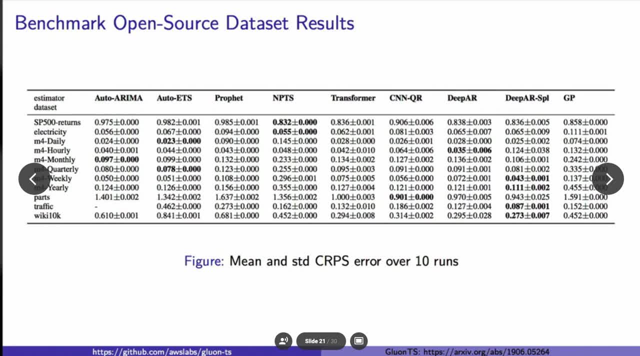 seasonal predictor which takes the past time point or past seasonal time point. We also provide transformer methods which are popular in NLP and use attentions, And then you'll see the sequence-to-sequence and canonical methods here, as well as the GP, And we see for different data. 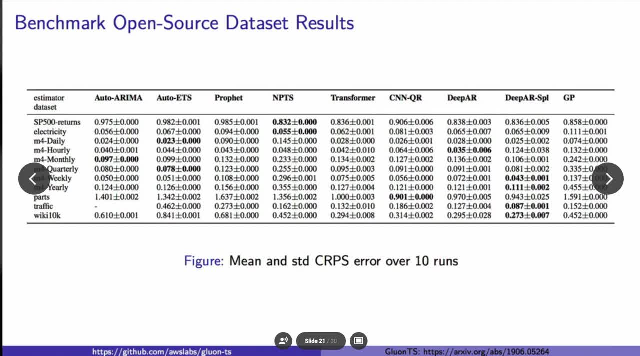 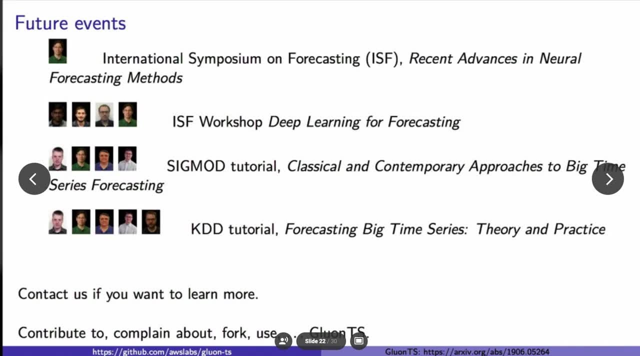 sets. different methods provide better accuracy And these results are averaged over 10 runs and we're plotting the mean And standard deviation. So I'd like to highlight other future events that our team is doing, So we'll be presenting at ISF next week, as well as doing tutorials on Glue-on-TS at Sigmoid and KDD. 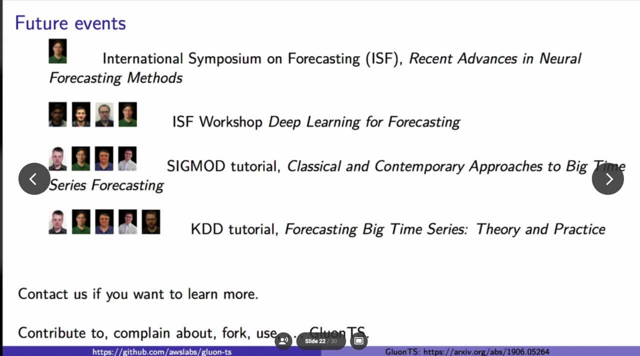 So contact us if you'd like to learn more. We have the GitHub link at the bottom And feel free to contribute to or complain about work or use Glue-on-TS. Any feedback is welcome for us, So we're really excited to have this open sourced. 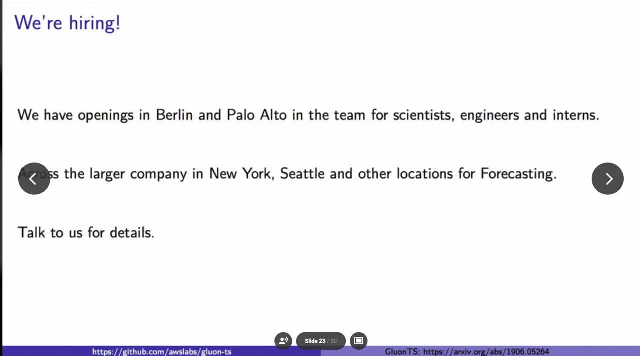 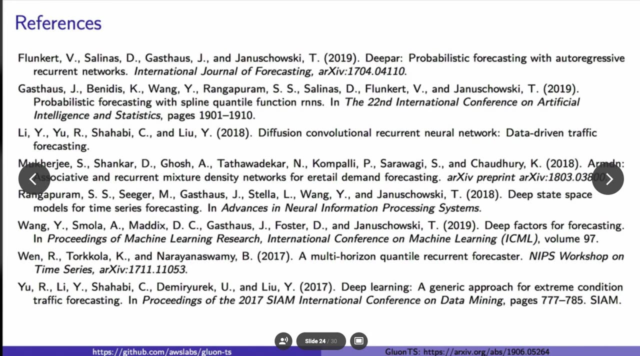 And, as a side note, we're also hiring, So we have openings in our Berlin and Palo Alto office for scientists, engineers and interns, as well as offices in New York and Seattle. So talk to us further for any details, And I've also provided references here since I went into the models. 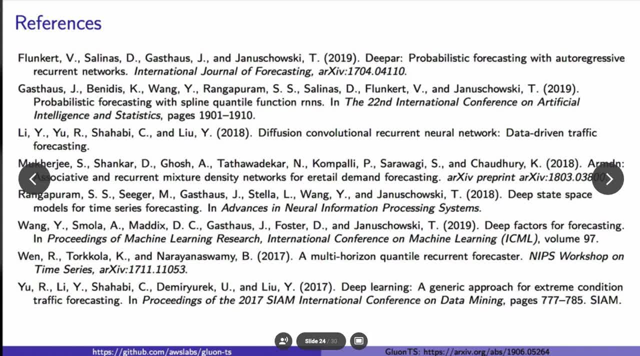 at a pretty high level detail. So if you want more details, you can see the papers here.